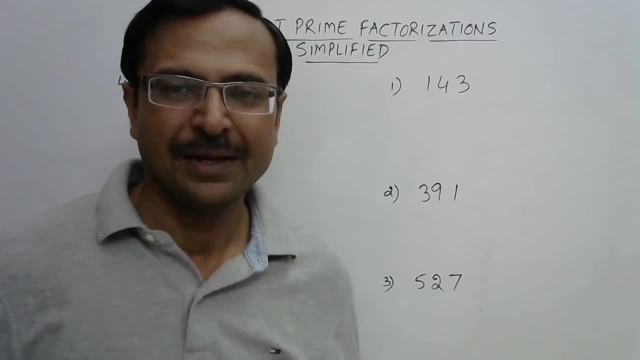 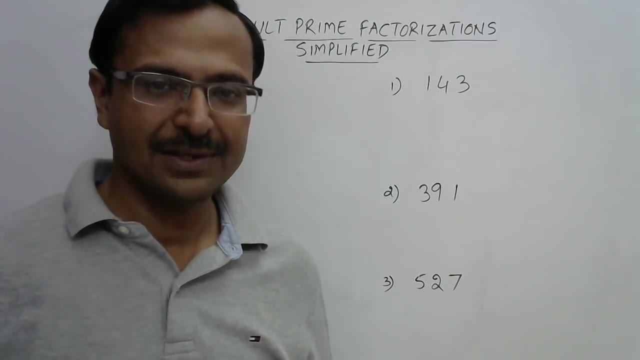 Hello, dear friends, Prime factorization: It can be a little bit tricky when the numbers involved in the prime factors are large. If you have a number which is divisible by 2, then anyone can make the prime factors. Or, for that matter, if the number is divisible by 3,, 5,, 7 or even 11,, students can make factors very easily. 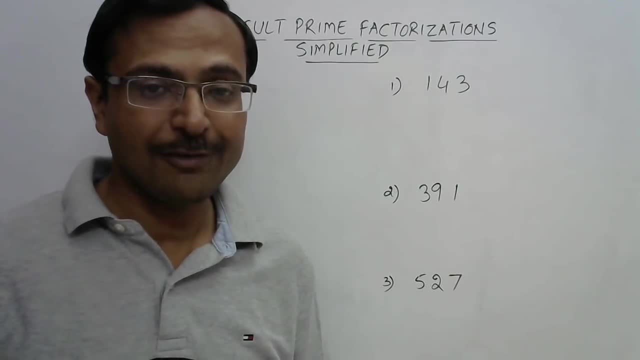 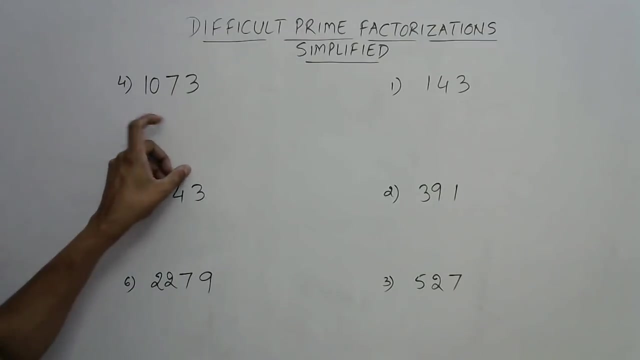 But if the numbers involve prime factors which are greater than 11, then students feel difficulty in making the factors of such numbers. Like you have the number 1073.. Now this number is not divisible by 2, not divisible by 3, not divisible by 5, neither by 7 nor by 11.. 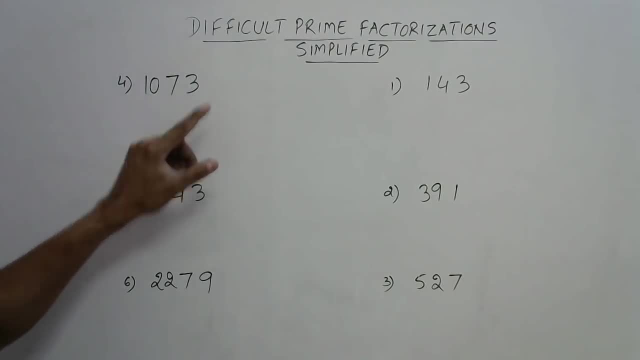 So making the prime factors is very easy, But making the prime factors of 1073 is difficult. So what option do we have now? Students can make prime factors of such numbers also easily if they have basic understanding of the prime numbers and their product. 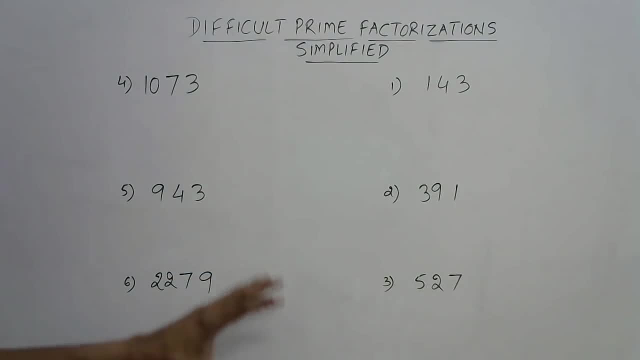 All these numbers which I have written here are product of two primes, And we need to find out which two prime numbers have to be multiplied in order to get the product of this number: 1073,, 943,, 2279, such large numbers- 2279. 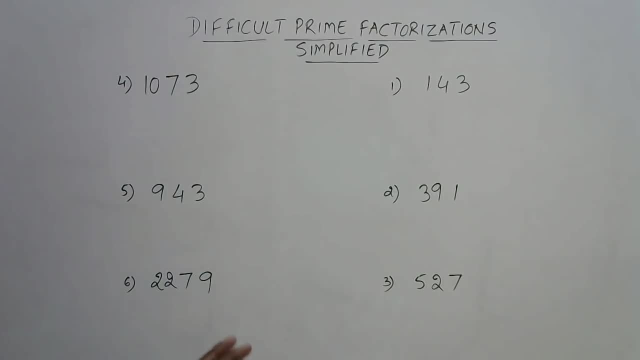 Most of the students cannot factorize this within 15 to 20 seconds. They will consume at least 1 minute or even more to factorize all these numbers. So I will take the basic example of 143.. And then we will try. 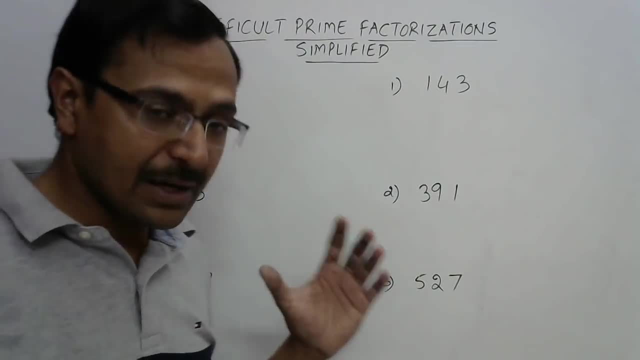 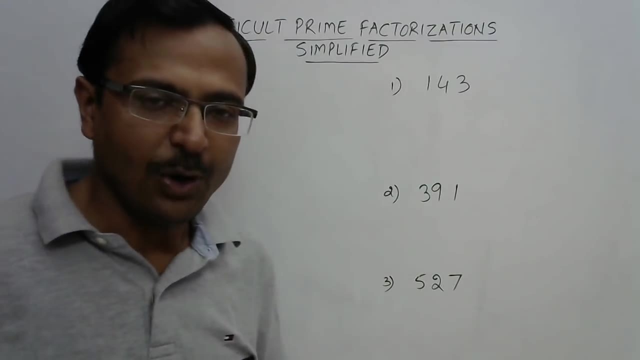 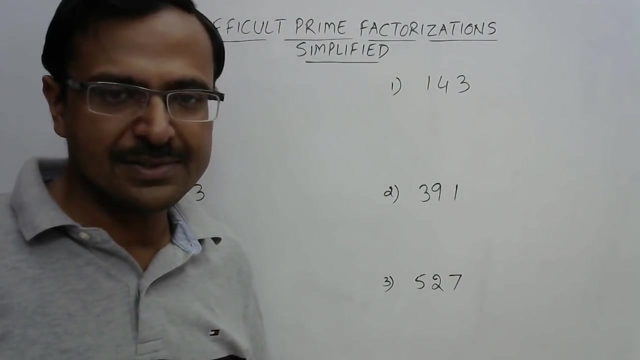 We can increase the complexity and try to factorize larger numbers which are product of two large primes. So let us develop the understanding of how we can get to this number Now. see 143.. The number is quite small And if you have to multiply two prime numbers then you cannot think of large primes like 31,, 37.. 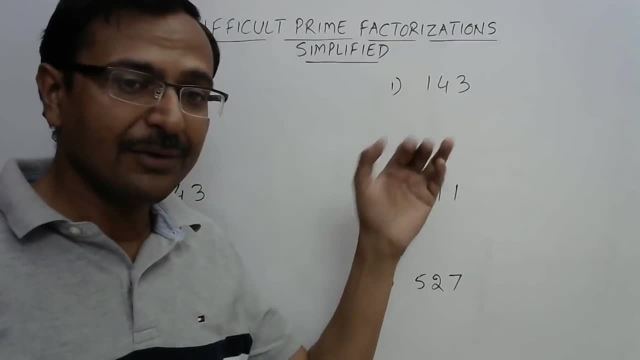 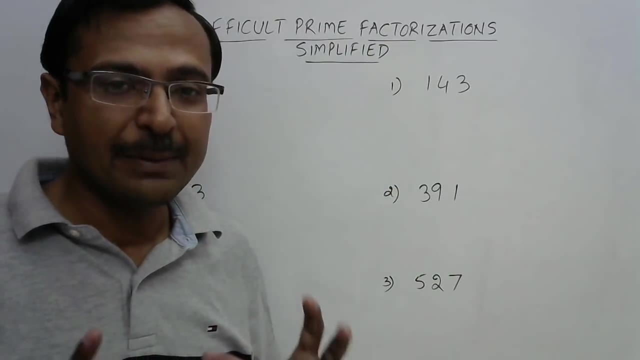 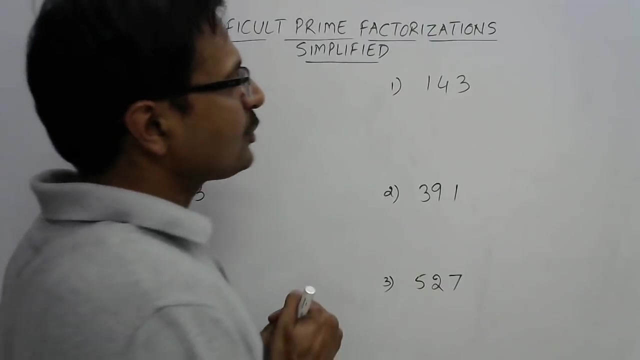 Why? Because their product with another large prime will be far more than 143.. So you have to think of prime numbers which are not above, say, 20.. If you see the unit digit here, that's the ones place. In the ones place, we have a 3.. 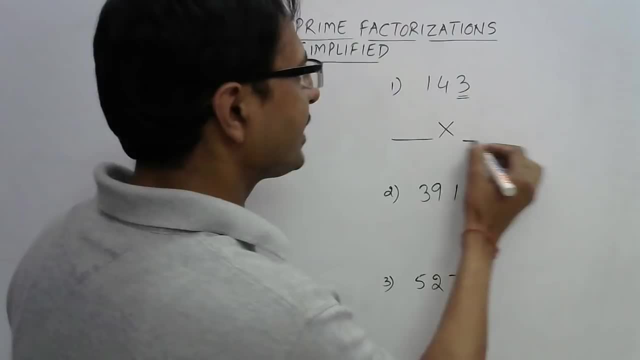 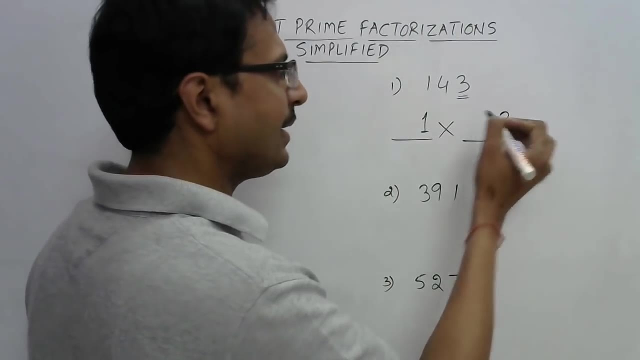 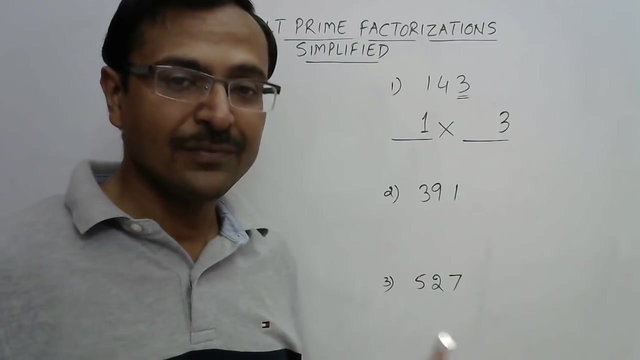 So if you want to have two prime factors whose product is 143,, then either the two numbers have to end with 1 and 3, because 1 into 3 is 3.. So the product of these two numbers may end with 3 and can give you a product 143. 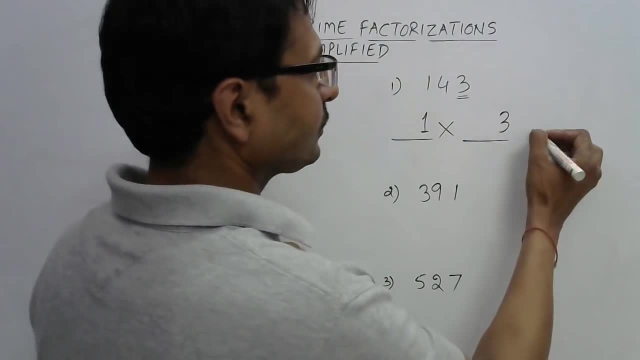 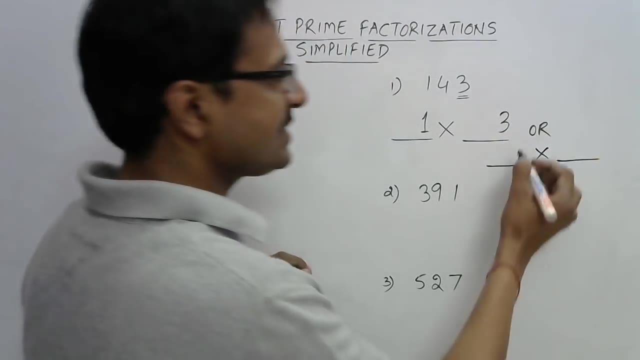 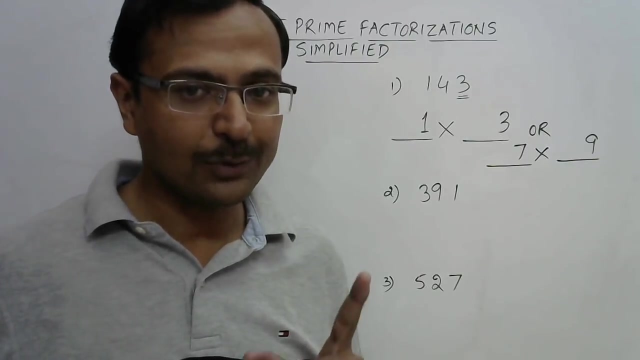 Or there is another possibility: You can have two numbers ending with 7 and 9.. The numbers ending with 7 and 9, if you multiply them, the product will end with 3.. 7 into 9 is 63.. 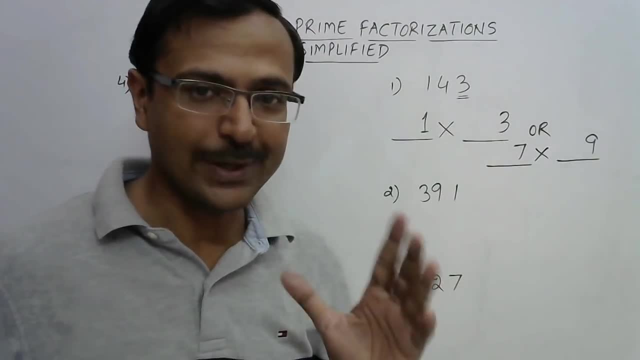 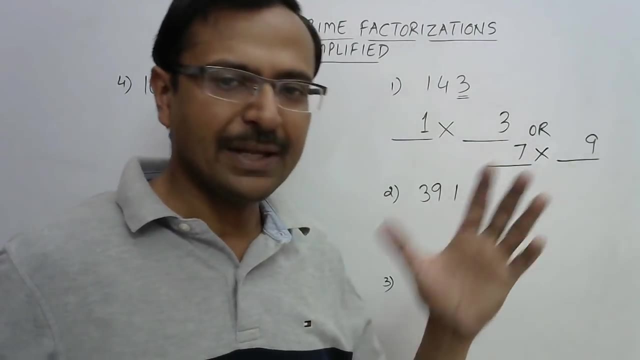 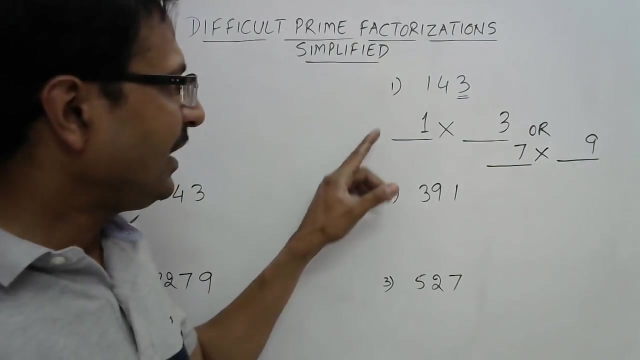 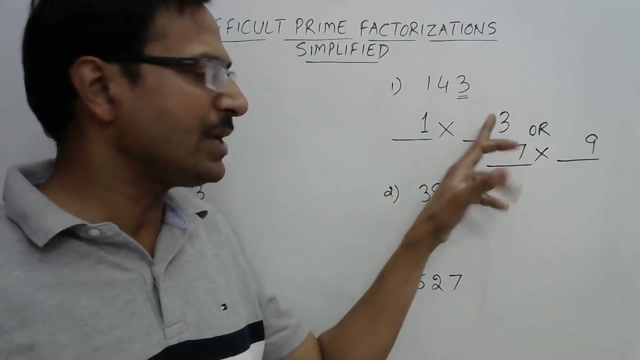 It ends with 3 and our number 143 is also ending with 3.. So these are the two possibilities. And now, if you have got to this step, then next step will certainly give you the correct answer. prefix 1 here this will become 11, and 11 into 3 is smaller than 143.. So if you prefix 1 here, 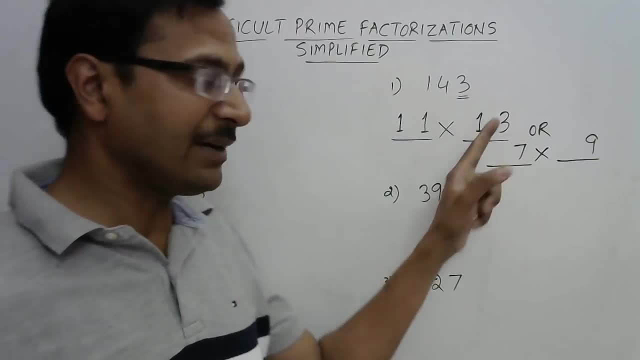 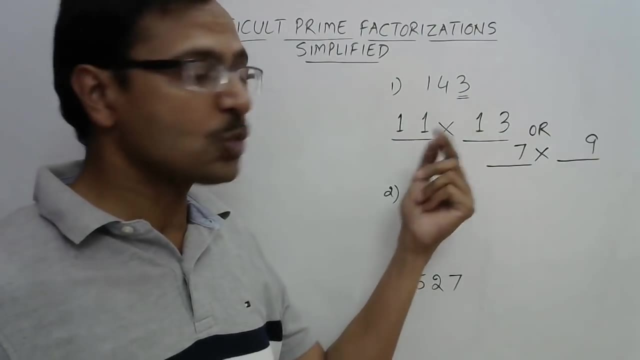 and 1 here. then both the numbers 11 and 13 are prime and if you multiply them your result will be very close to 130, because 13 into 10 is 130.. So 13 into 11 is going to give you 143.. 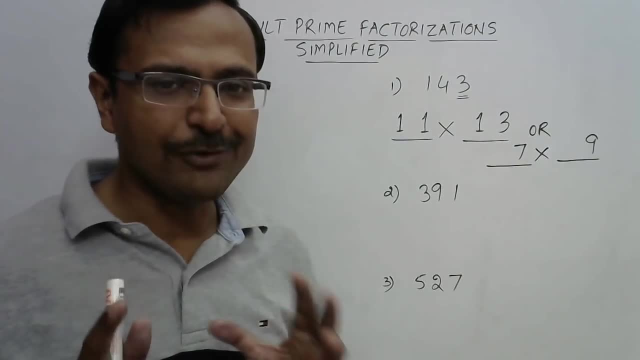 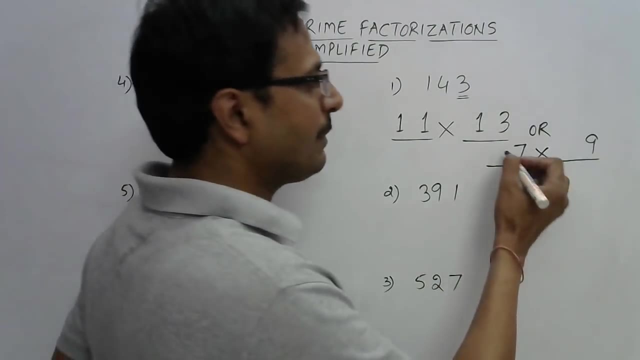 So 143,. the prime factors are quite obvious. just by little bit of understanding, You do not need to test 7 and 9.. Why? Because if you multiply 17 and 9, you cannot do it because 9 is not prime. 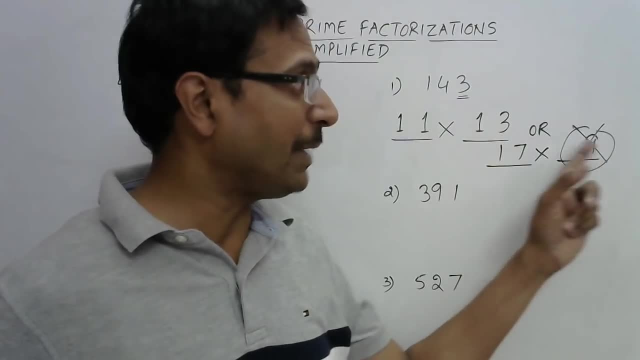 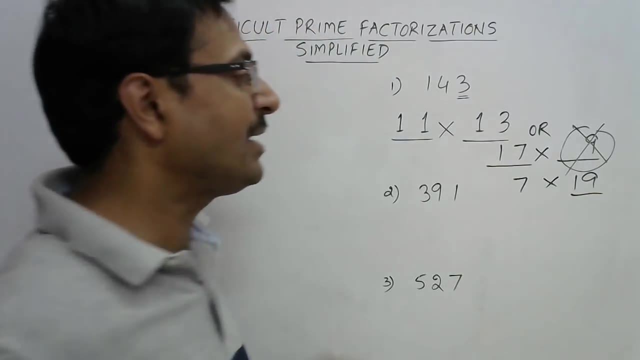 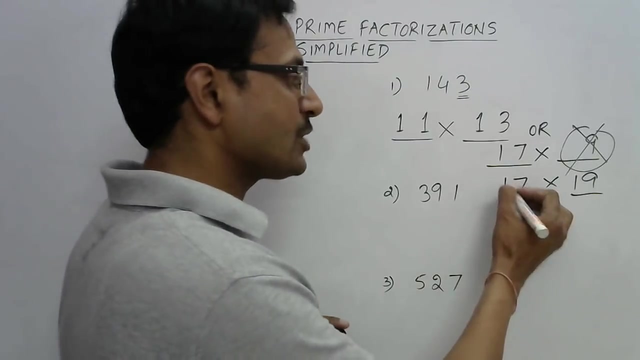 So you cannot take 9.. So you have to prefix 9 by a number. and if you prefix 9 by 1, it becomes 19 and this becomes 7.. Then 19 into 7 is not 143.. So if you prefix this also by 1, then it becomes much, much larger than 143. 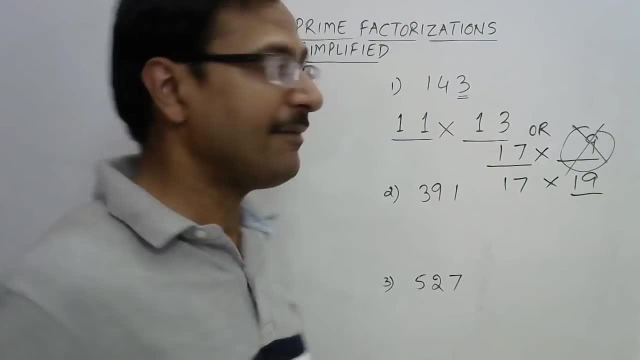 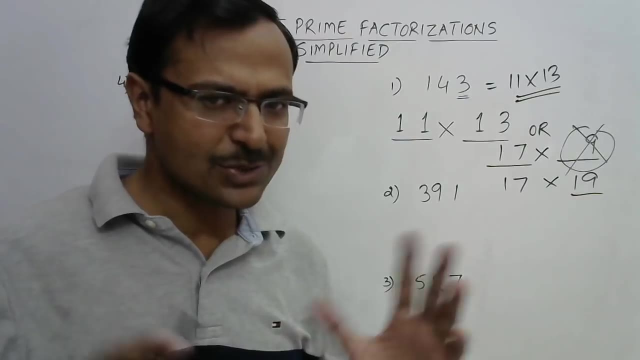 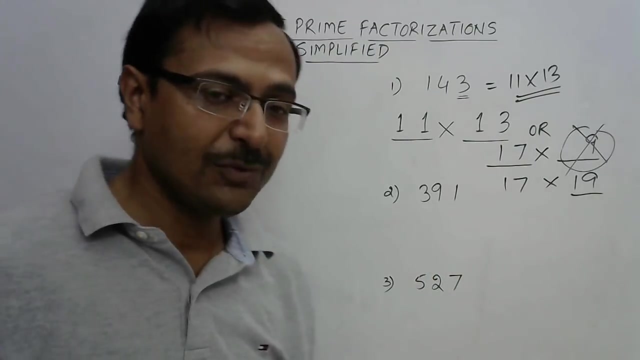 So your obvious answer for this question is 11 into 13.. So even if you have understood 20 percent of this, it is fine, because we are going to solve 5 more problems based on this method of factorizing a large number which is product of 2 primes. So 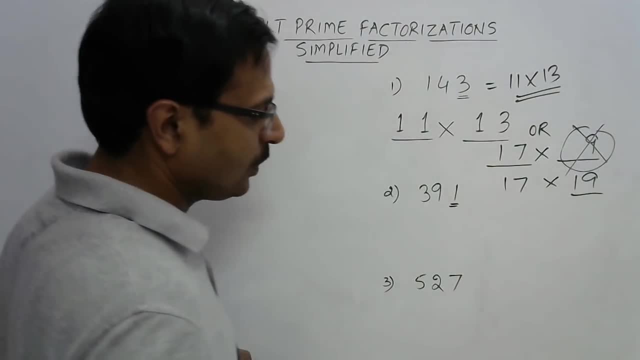 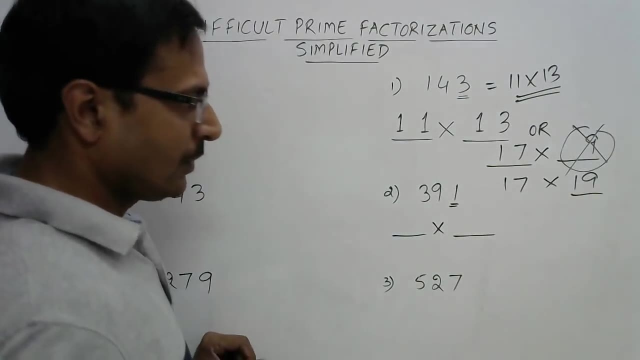 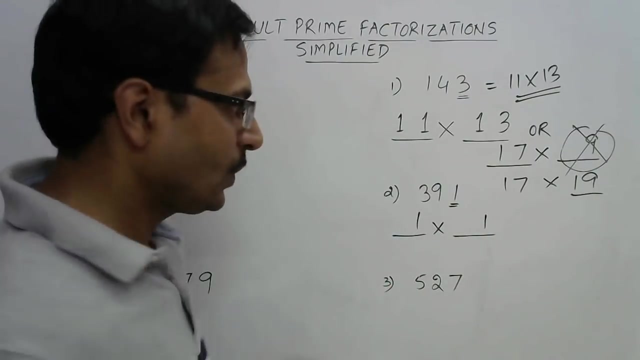 let us start with the first problem. The first problem is: what is the number that is ending with 1?? Now see the number is ending with 1.. So what are the options? You may have 2 numbers. See the product is 1.. So both the numbers can end with 1, because 1 into. 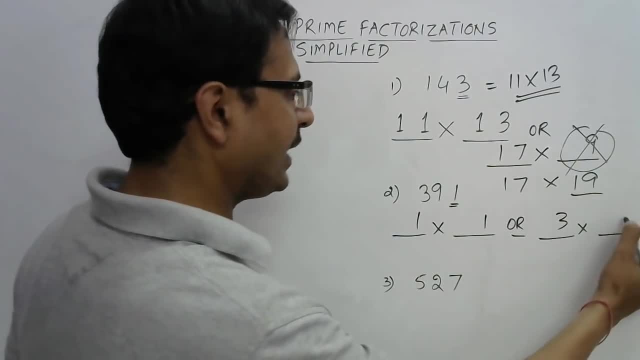 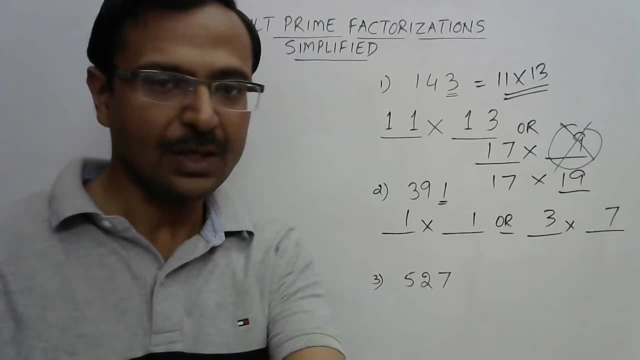 1 is 1, or you may have 2 numbers, 1 ending with 3 and 1 ending with 7, because 3 into 7 is 21,, which again ends with 2. 1. So these are the two possibilities. Now let us look into it, See if I write 1 here. 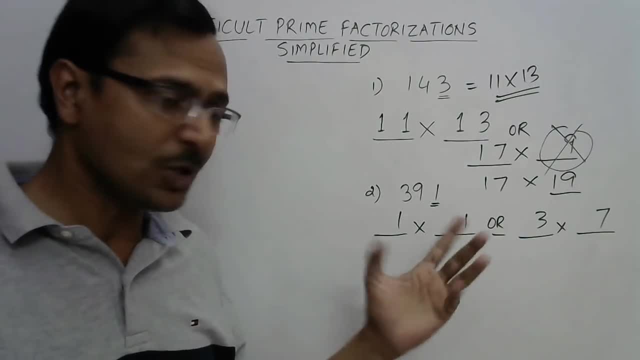 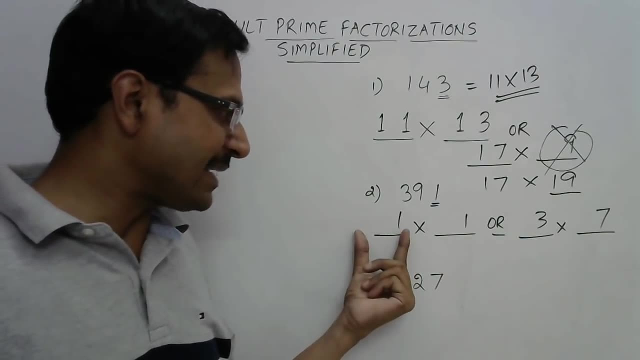 11 into 1 is very less than 391 and 1 is not prime, So you have to prefix a number in both these. So if you make this 11 and 11,, 11 into 11, is 121, which is again less than 391.. So 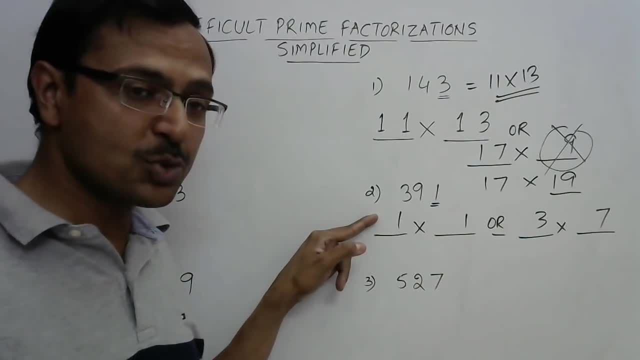 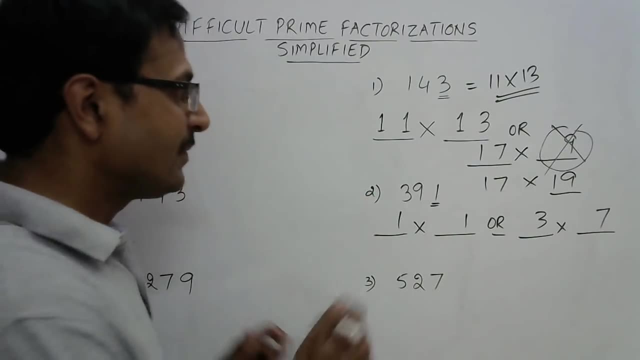 you have to get on with this increasing it. If you prefix 2, then 21 is not prime, So you cannot prefix 2.. You can prefix 3.. Why? Because 31 is a prime number and 11 is also a. 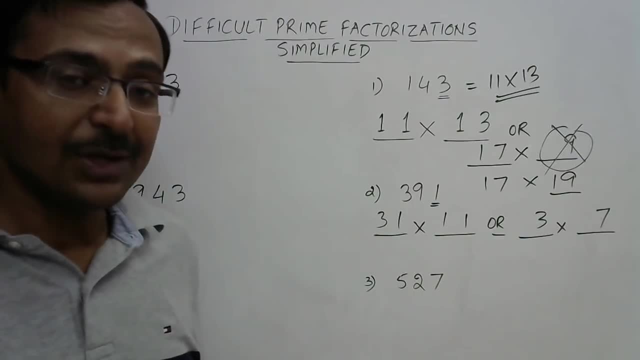 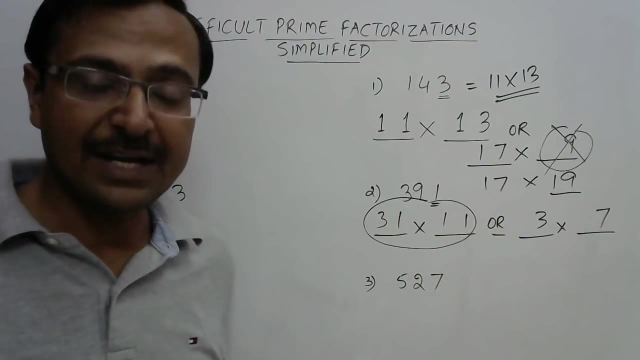 prime number, But 31 into 11 is not 391.. So if I go beyond this, then this will be greater than 391.. So there are very few possibilities that our answer will end with 1 each. So what are options we have? 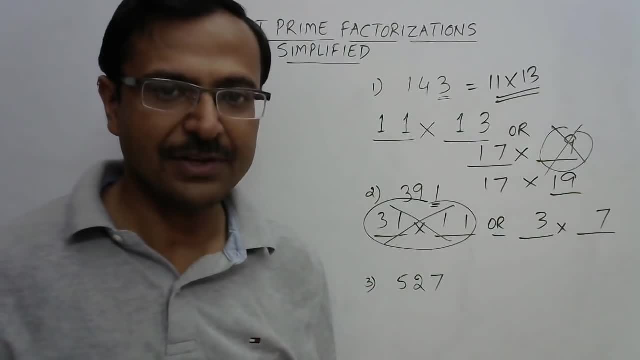 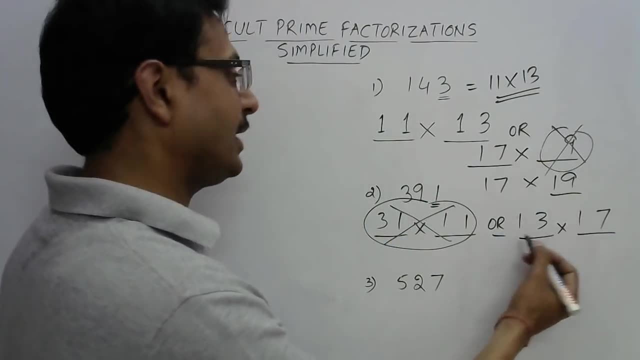 We have 3 and 7.. Now let us try with 3 and 7.. If you prefix 1 here, 13 into 7 is not 391.. If you prefix 1 here, 13 and 7, both are prime, But 17 into 10 is 170.. So this is not going to. 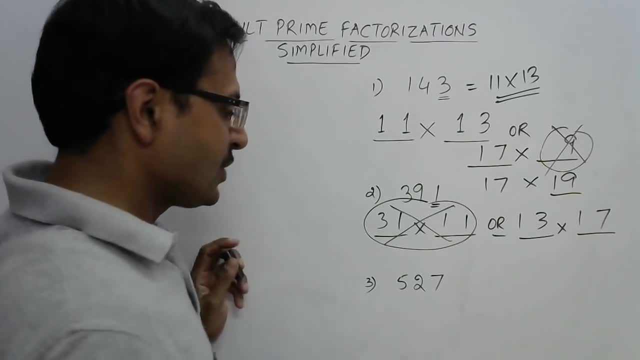 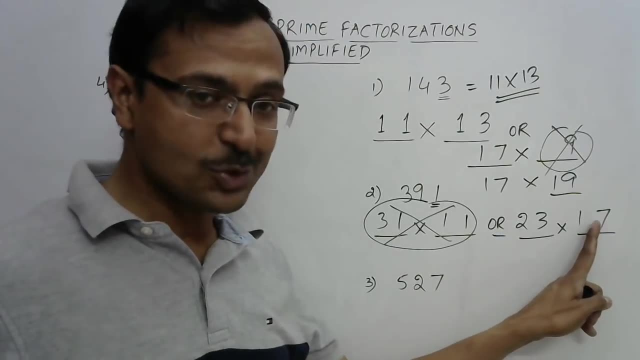 give me 390. So I need to increase it. So suppose I increase this by 2.. Now it gives me 23, which is prime, But 27 is not prime. So I have prefixed 2 here. So 23 into 17,. 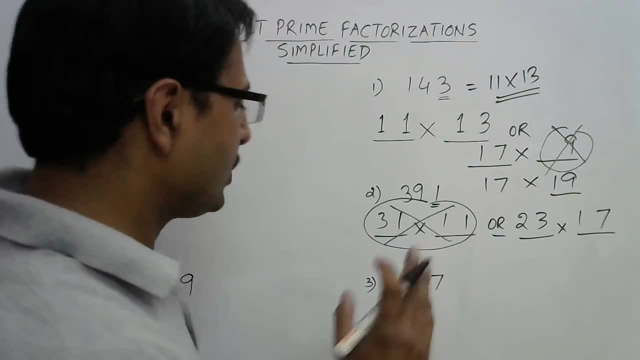 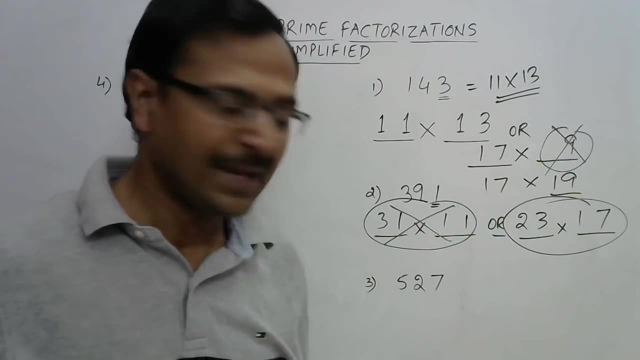 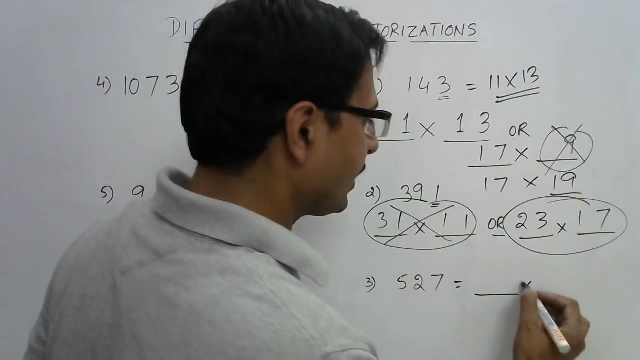 just try this out: 23 into 17 is going to give you 391, which is the prime factorization of 391.. Let us see 527.. Now again, the unit digit is 7.. So what options we have? So either the number, 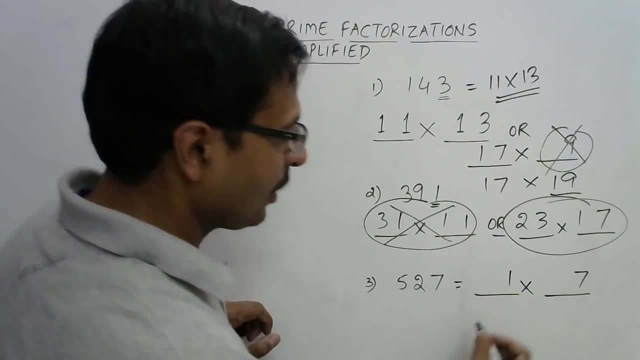 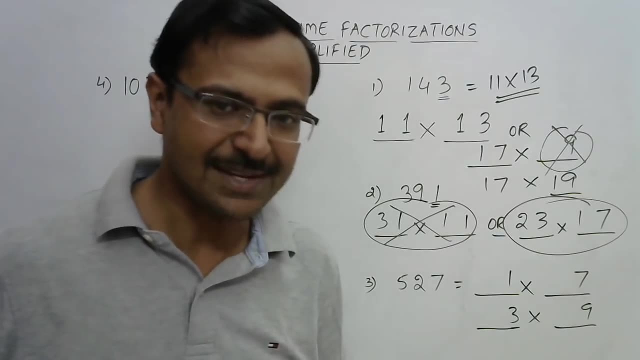 will end with 1 and 7, because 1 into 7 is 7, or the number will end with 3 and 9, because 3 into 9 is 27, which ends with 7.. So let us try 1 and 7.. 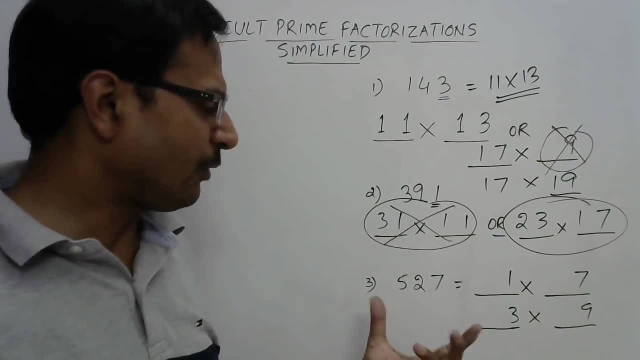 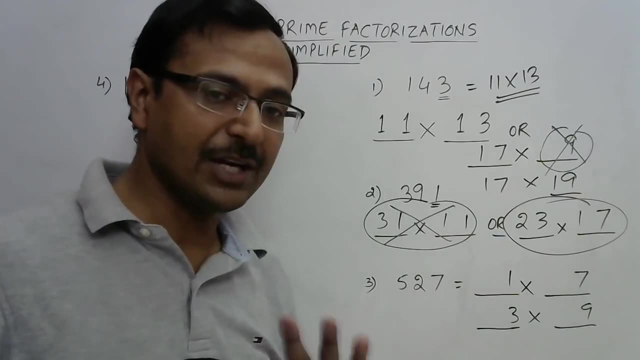 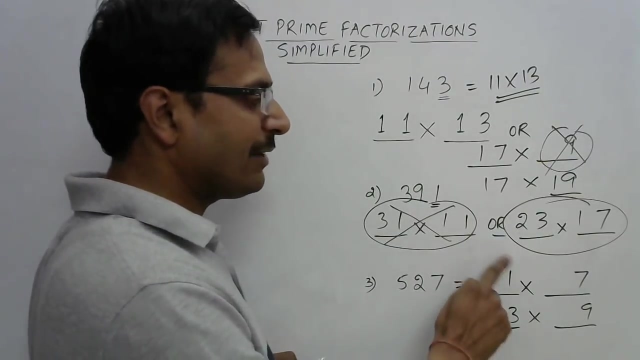 See, I will straightforward move to 20s and 30s. Why? Because 10s, 11,, 17,. they are not going to give me 527.. Let us try with 20s. If I take 2 here, this is 21, which is not prime, So I cannot. 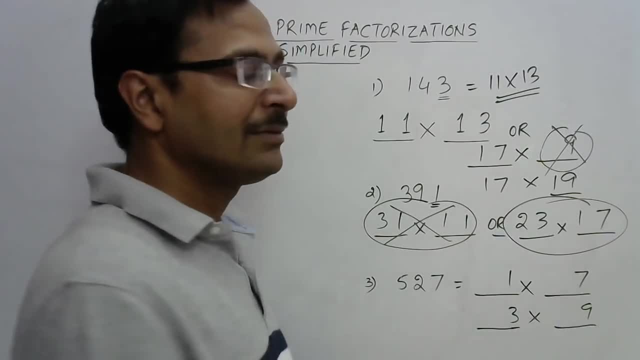 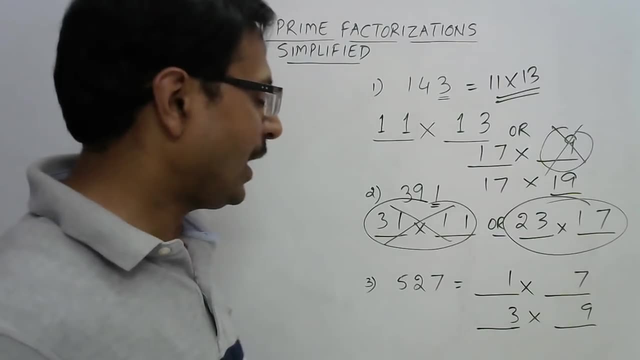 have 21.. If I take 2 here, this is 27.. 27 is also not prime, So I cannot go with 2s in both the numbers. So I will have to go with 2s. So I will have to go with 2s. So I will have to go with 2s. 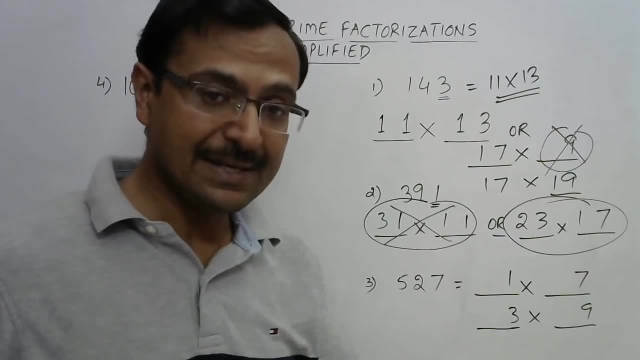 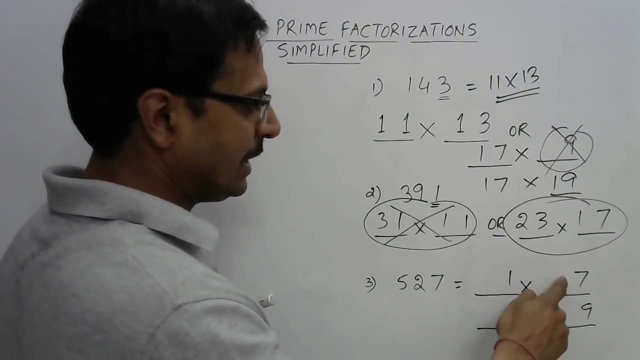 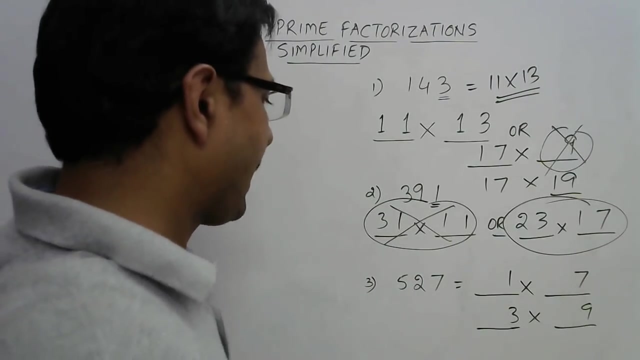 So I will either stay in 10s or go in 3s. Now, if I move in 10s, 11 into 7,, 11 into 17,, these are not 527. It is a large number, So let us have some other number. 11 is not going to. 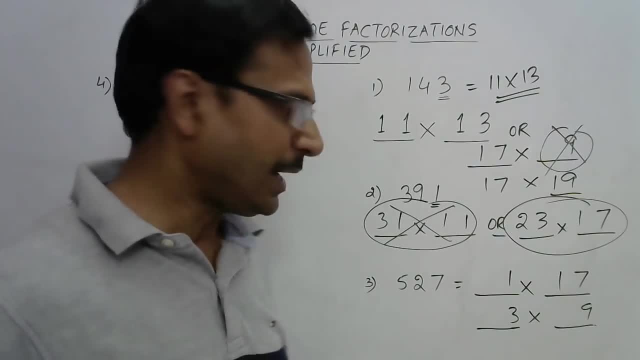 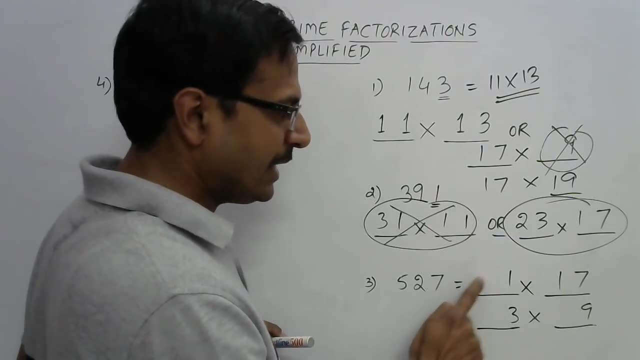 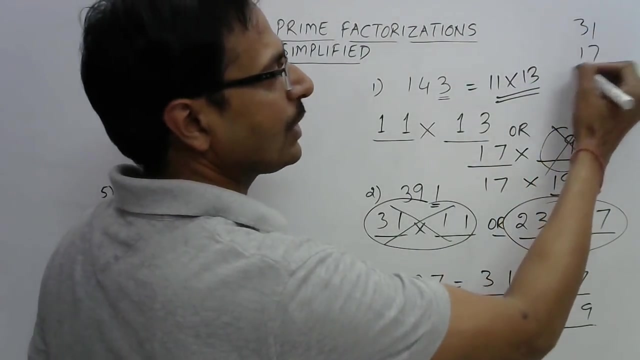 give me 527.. So let us have 17 here and write with 11, 17 into 11, again 187.. So very less number 21 I cannot take, So let us take 31.. Just try 31 and 17.. 31 into 17,. you can use the. 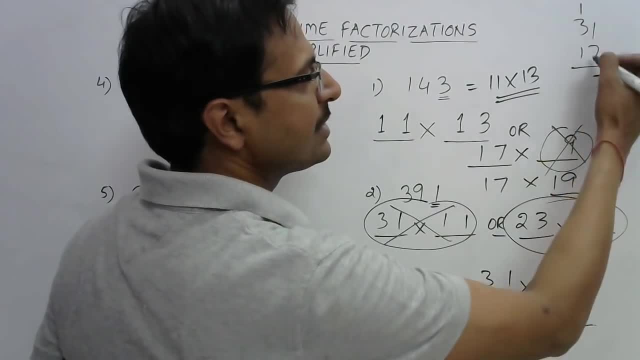 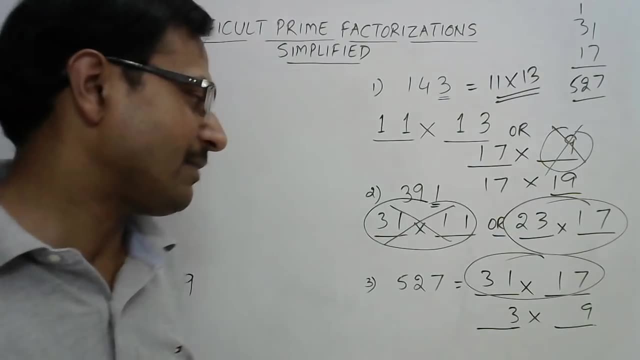 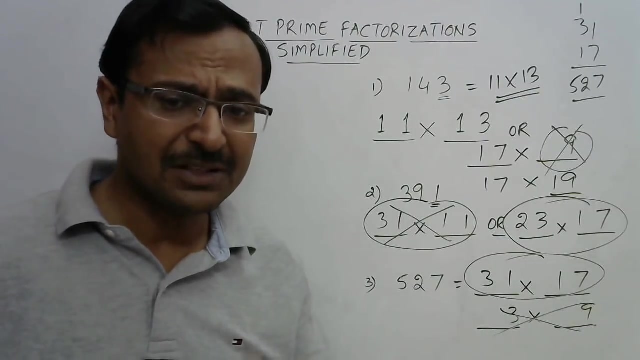 basic method or you can do directly: 17 into 1 is 17.. 17,. 3 is a 51 plus 1, 52. So 527.. Exact factorization of 527, 17 into 31.. So you do not need to consider 9 and 3s Students the method. 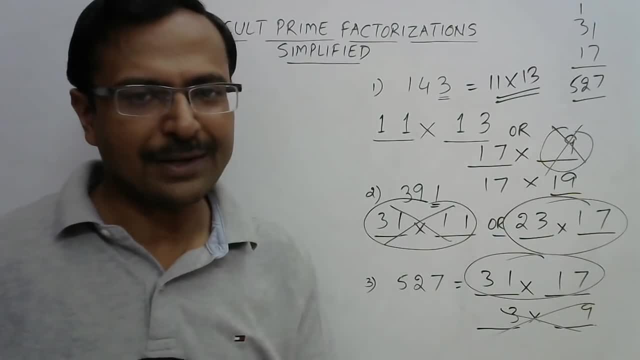 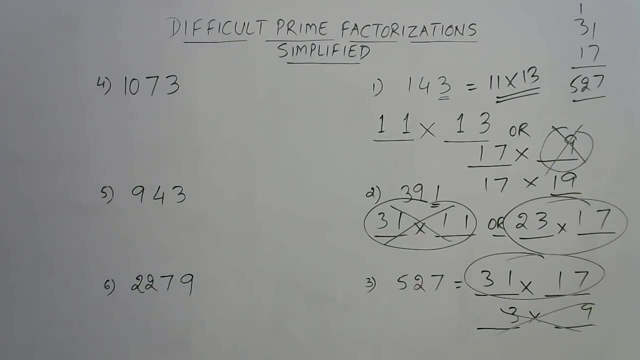 might feel little bit difficult for you, But little bit of practice and I am sure you are going to factorize numbers in thousands like this very, very easily in a matter of just 10 to 15 seconds. So just consider 1073.. See, we have a 3 here, So our number is going to end with 1 or 3. 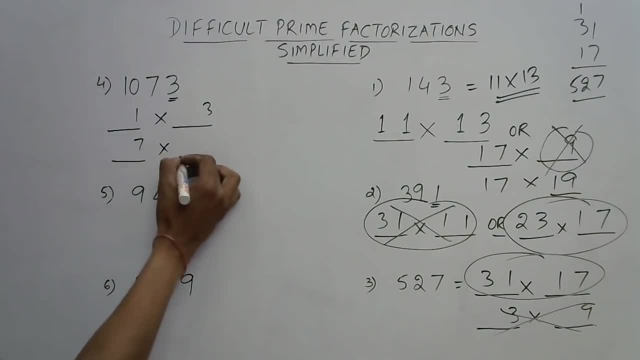 and the other option is 7 and 9.. So there are only two possible options. We cannot have even numbers here. We have to end with 137 and 9 only Now. 1073 is quite a large number. So I need to think of 20s and 30s, 40s like this. So let us go. 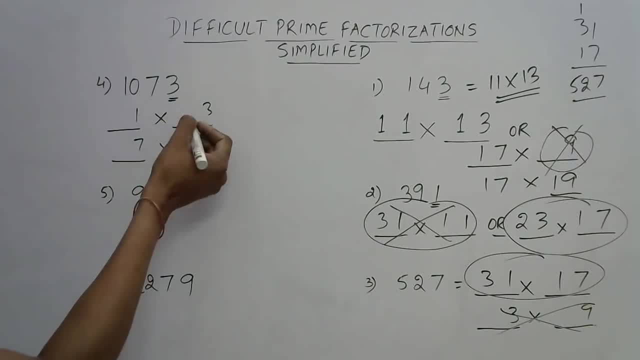 with 1 here. 11 into a two-digit number is not going to give me a number in thousands, So let us go with 2.. 21 is not prime, So I cannot have 21 here. I can have a 23 here and 11, not 1073, 21,. 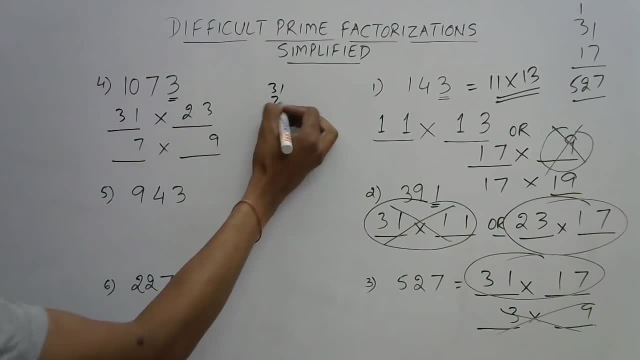 no 31. So 11 into 23,, 30 into 2600. So that is quite less than this. So no option Here you can have 41.. 40 into 20 is 800, again quite less. No, So go with 51. So let us see 51 and 23.. 23 into 1 is. 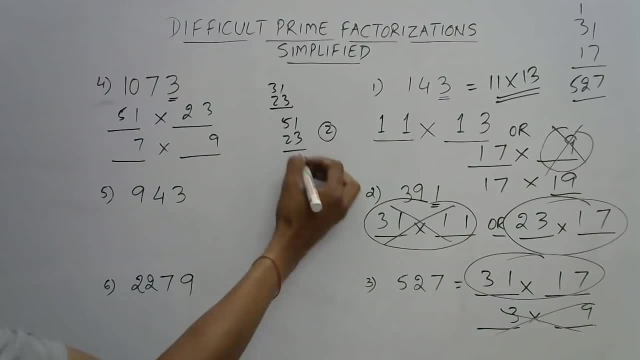 23.. So 2 carry 23 into 5 is 115, 118. So that is quite large. So this option nearly stands cancelled. Now think of this. Single digit into a double digit is not going to give me thousands. Okay, I can have a 17 and a 19.. 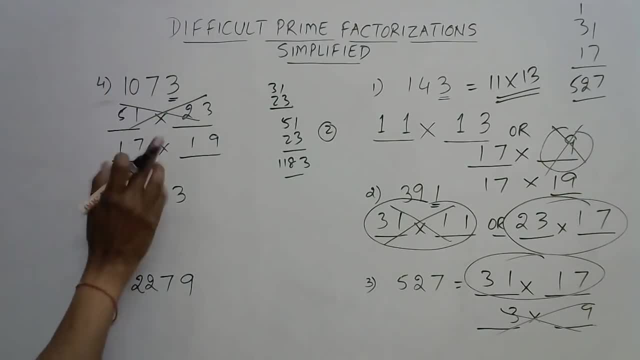 20 into 20 is 400. So this is going to be less than 400.. No, not an option. I can have a 29 here. 29 into 17,. 30 into 17 is 510, again less. So we can have a 3 here, 37,. now test 37 and 29.. 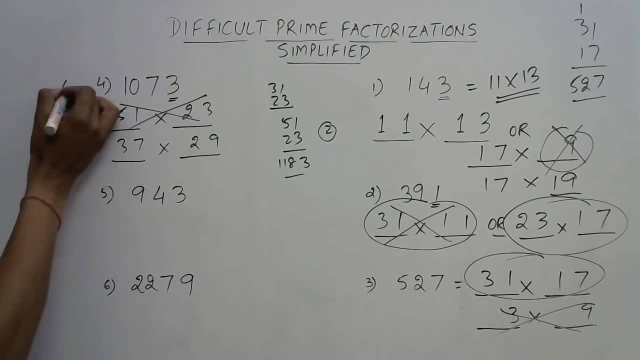 37, 29.. 29. So 79 is 63.. So 6 carry 27 and 14 is 41.. 6 is 47. See 4 carry 6 plus 4, 10. So 1073.. Same number. So here we have the prime factorization. 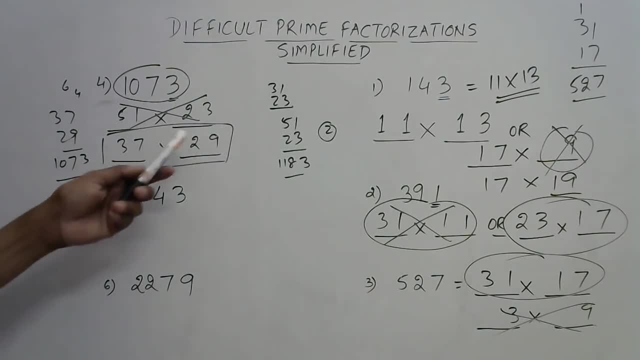 of 1073 as 57 into 29.. 943, again 1 and 3.. See again. we can make use of 11 into see 23.. No 43 into 11, again very much less. 53 into 11,. 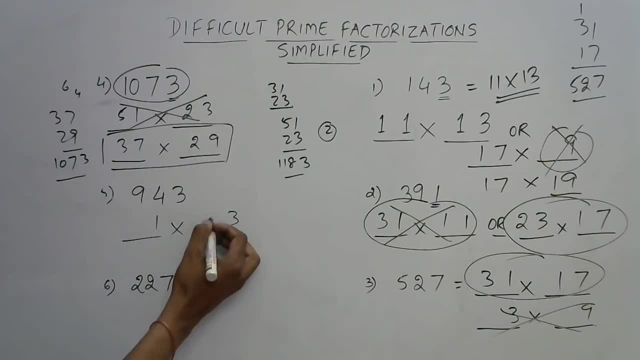 583, no 63 is not prime. 73 into 11, again less 83 into 11.. So 83 into 11. 11 is equal to 33.. 3, 11 is 88, 91. So that's quite close, But it is not giving me the correct answer So I cannot. 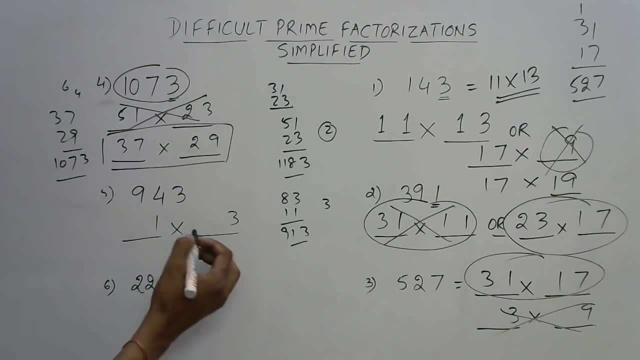 increase this, So let's increase this one now. Okay, I'll have. 11 is not going to give, 21 is not prime 31 and suppose I have. let's say, 11 is not going to give, So let's increase this one. 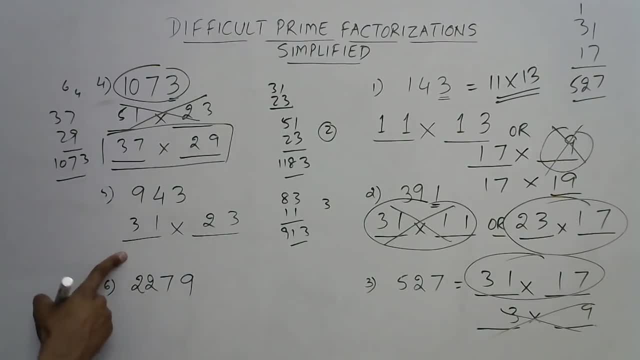 I have here 23.. This is 600.. No, So let's increase this: 41 and 23.. So 41 and 23.. 3 and the 3.. So this is 12 plus 2,, 14,, 4, 1.. So 8 and 1, 9,, 9, 43. That's the great method. 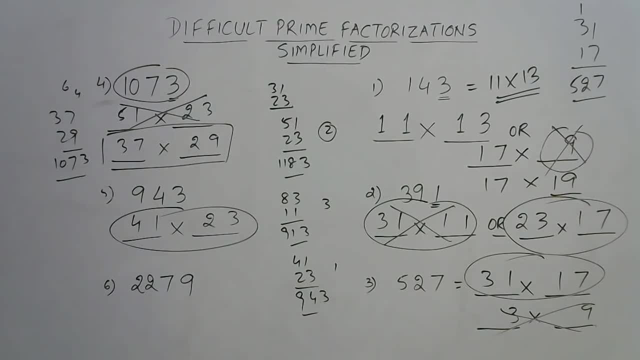 which has given us the correct factorization of this also. Finally, we have doubled 7, 9.. So either the number is going to end with 3 and 3. And the other option, it can be 1 and 9.. So you can try with this And you can get to the answer. This is more than 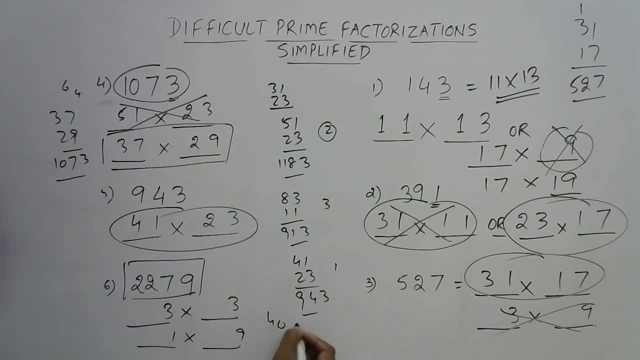 2000.. So our number has to be in 40s, 50s, Because 40 into 50 is 2000.. So if you try with 4, you have 5 here, 43 into 53.. Just try it, Your answer will be doubled to 7,, 9.. So this is.